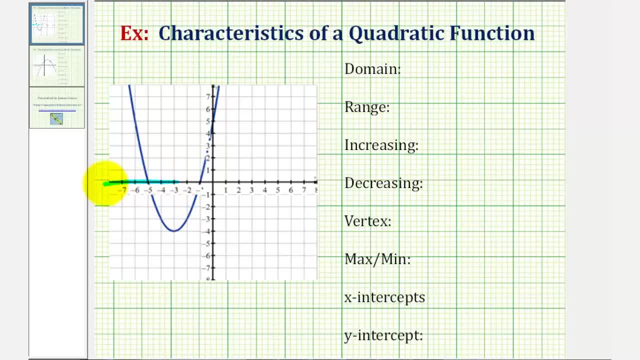 onto the x-axis. it would move to the left forever and move to the right forever And therefore the domain would be all real numbers, which is a domain for all quadratic functions. We can express this several ways. Using interval notation, we'd have the open interval. 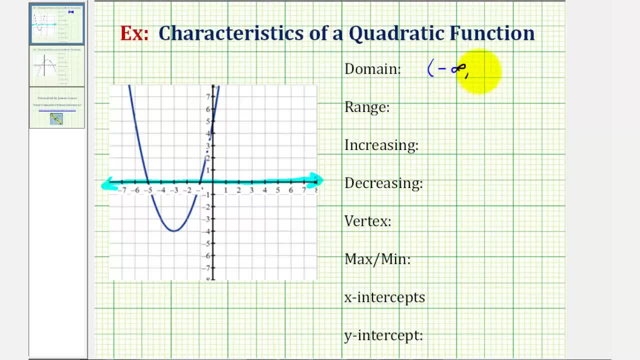 from negative infinity to positive infinity. Of course we could also say x is greater than negative infinity and less than positive infinity. These two are equivalent. The range is a set of all possible y values And since the y values run along the vertical axis, 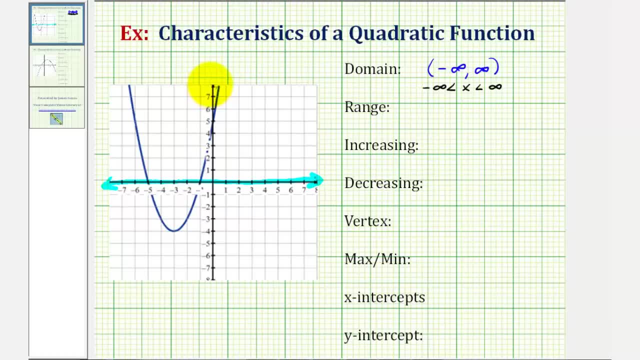 we can think of projecting this onto the y-axis, Or notice how the lowest point on this graph is at the vertex where the y value is negative four, And then from negative four, the y values increase without bound. Therefore, the range would be the interval. 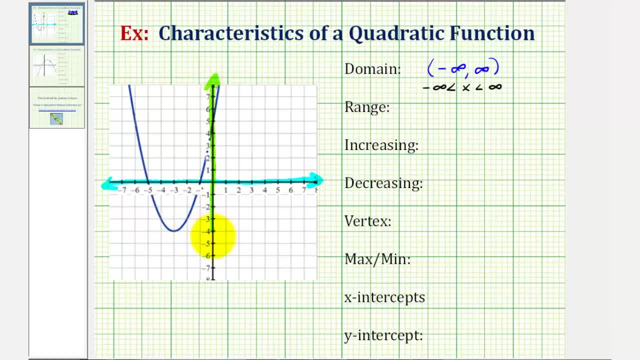 from negative four to infinity, Closed on negative four because it does include negative four. So, again using interval notation, we can say the interval that's closed on negative four to positive infinity. Or, using inequalities, we could just say y is greater than or equal to negative four. 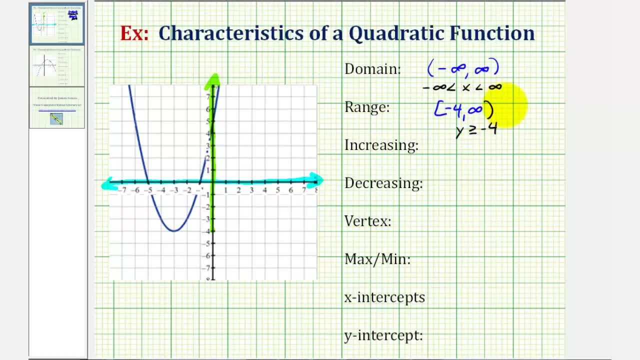 Again, these two are equivalent. Next, we're asked to determine when the function is increasing and decreasing Informally. if we walk on the graph from left to right, if we're going down to the left, if we're going downhill, the function is decreasing. 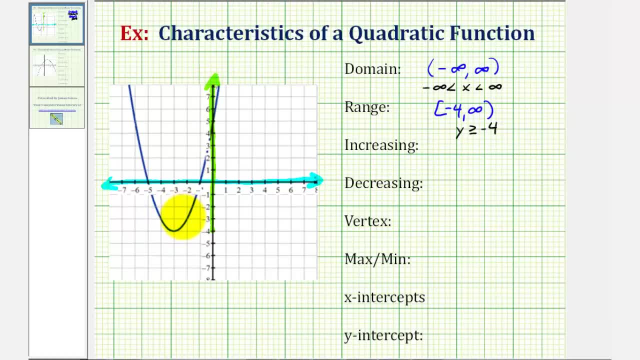 If we're walking uphill, the function would be increasing Again when walking from left to right. More formally, if as x increases, y decreases, the function is decreasing. And if, as x increases, y increases, the function is increasing. 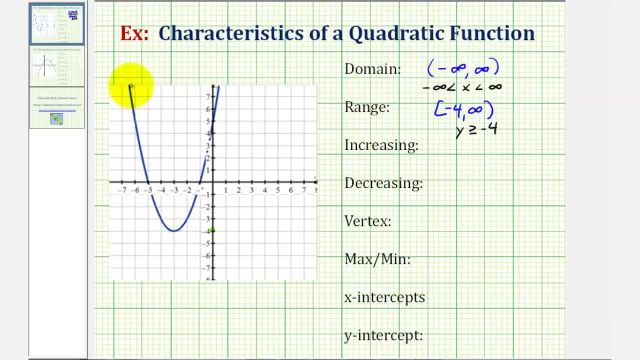 So, looking at the graph of our function, notice how, on the left of the vertex to the vertex, the graph would be decreasing, And to the right of the vertex the function is going uphill or increasing. When giving the interval for which the function 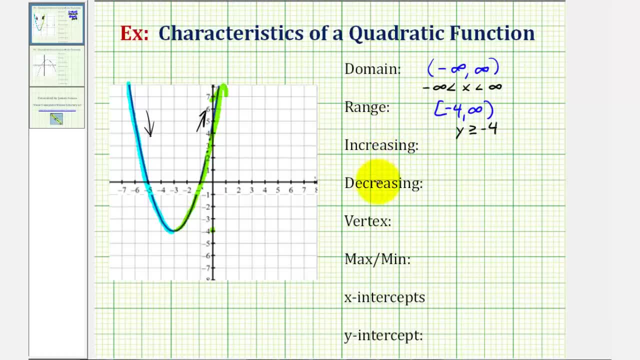 is increasing or decreasing. we want to use x values, So notice how the x value of the vertex is negative three. So the function would be decreasing on the interval from negative infinity to negative three And it's increasing on the interval from negative three to infinity.